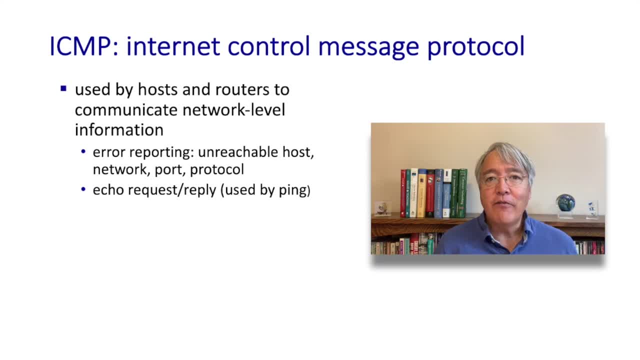 network-level information to each other. Often this information is in the form of error reporting, for example, a network or a host or a port or a protocol that's unreachable. An ICMP messages are also used in ping and traceroute. ICMP messages are carried directly as payload. 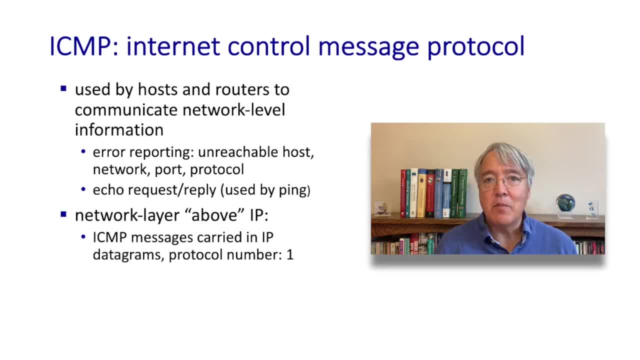 inside an IP datagram, just like UDP and TCP segments are carried as payload inside an IP datagram. So in that sense we can think of ICMP as a sibling protocol to UDP or TCP, but we really won't think of it as a transport layer protocol. As an upper layer protocol, ICMP also has a 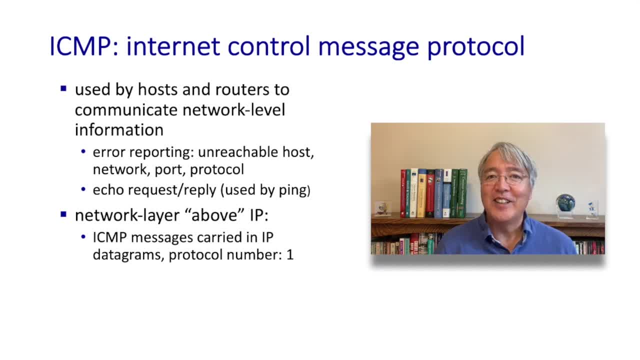 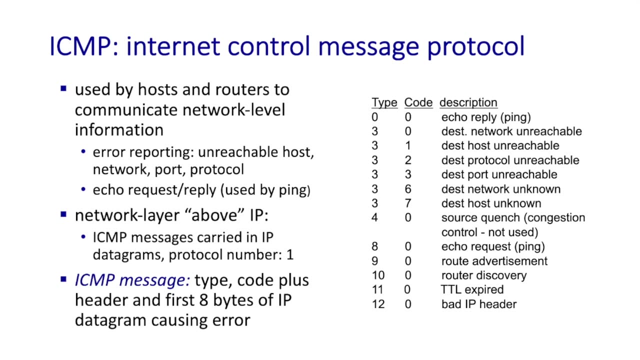 protocol number. Its protocol number is 1.. It's the number that's going to be used to connect to the very first number And, as you remember, this protocol number is used for demultiplexing up from IP, whether it be to ICMP, to UDP or to TCP. An ICMP message has a 1-byte type field, a 1-byte. 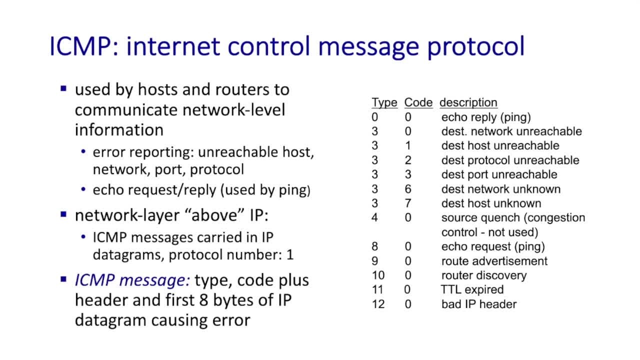 code field, a 2-byte checksum field, and then the header and up to 8 bytes of the IP datagram that caused an ICMP message to be issued in the first place. For example, it might contain the first time the TTL was exceeded. You can see the type and the code field shown here. You might note that. 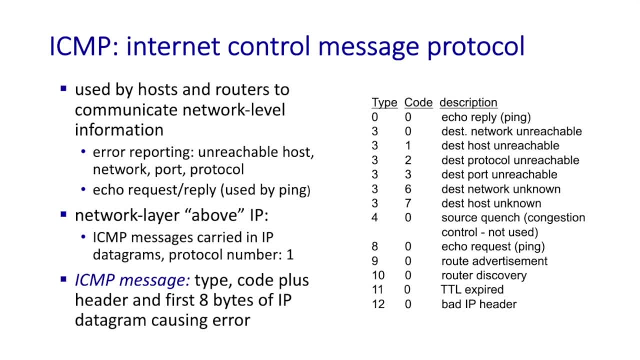 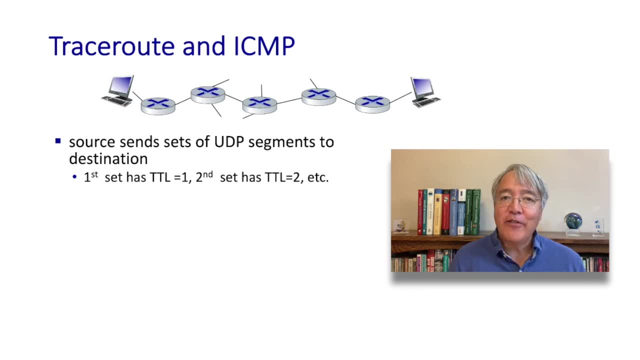 type 11. code 0 is the ICMP TTL expired message, which means that a router's received a datagram decremented the TTL field and the TTL field is now 0. This message is going to be key to how traceroute works Well. with this as background, you can probably already figure out how the 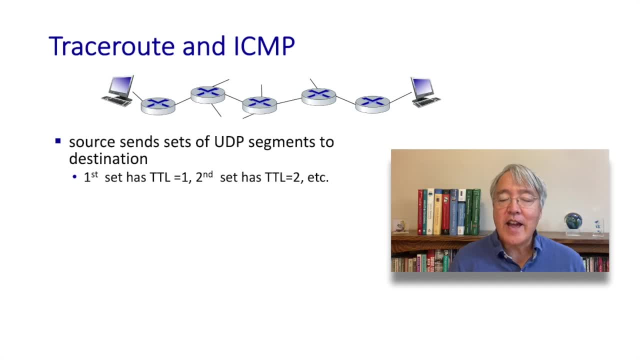 traceroute program works. Traceroute works by sending a set, usually a set of three UDP datagrams towards a destination. The first set of datagrams is sent with an IP TTL field value set to 1.. The second set is sent with a TTL value of 2.. The third is sent with a TTL value of 3,. 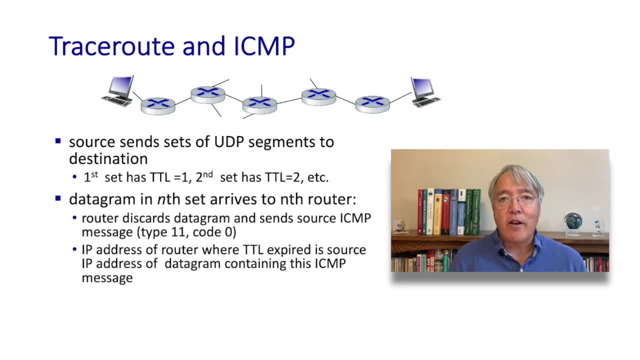 and so on. Now remember an IP router: when it forwards datagrams, always has to decrement the TTL field, And when that TTL field is decremented to 0, that datagram needs to be dropped at that router. That router may.